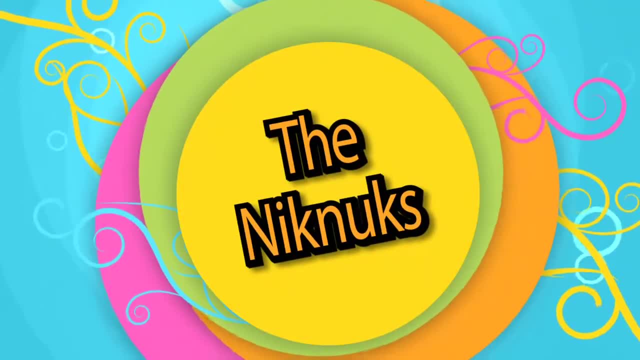 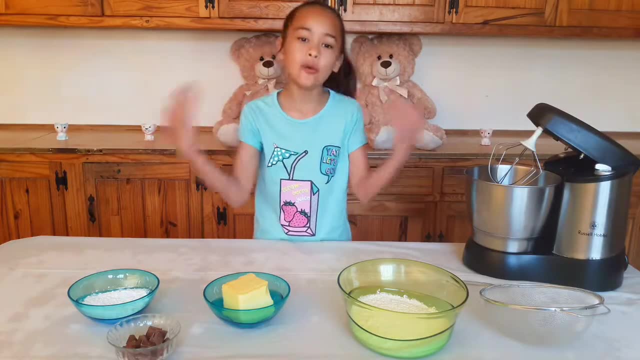 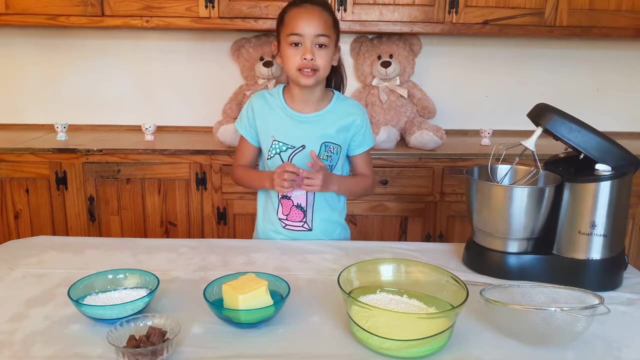 Hey guys, welcome back to the MakeMix channel. It's me Karanak once again, And today I'm going to be doing another baking video. Today I'm going to be teaching you guys how to be making some biscuits. Three ingredient biscuits, Very easy. 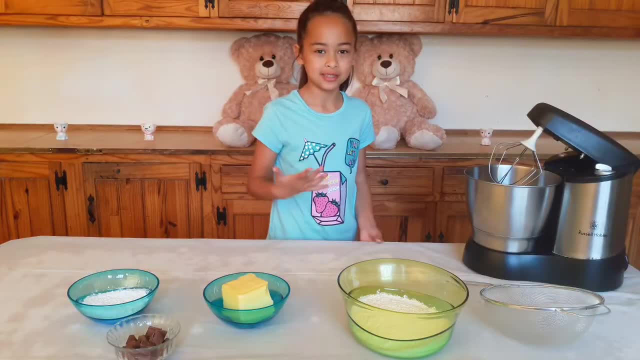 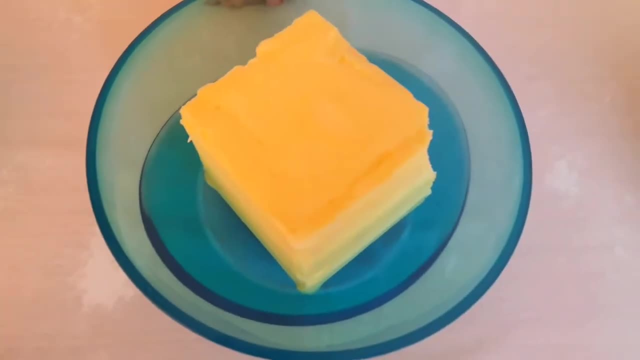 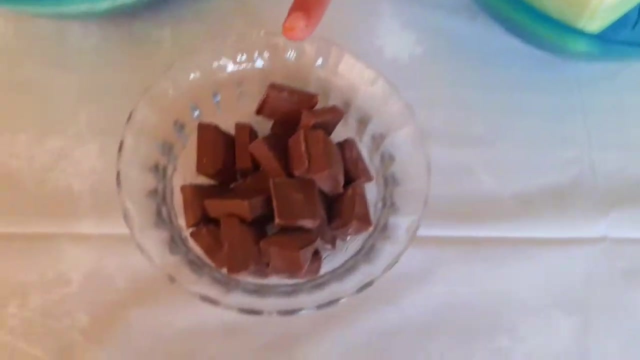 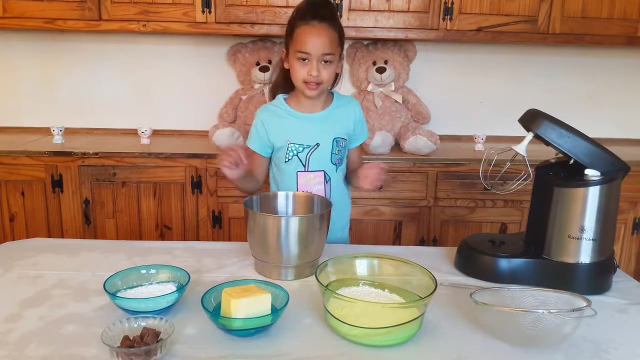 Okay, guys. so you'll need for this biscuit a half a cup of icing sugar, one cup of butter, two cups of flour, And the chocolate over here is optional. You'll need to heat your oven up to 180 degrees Celsius. 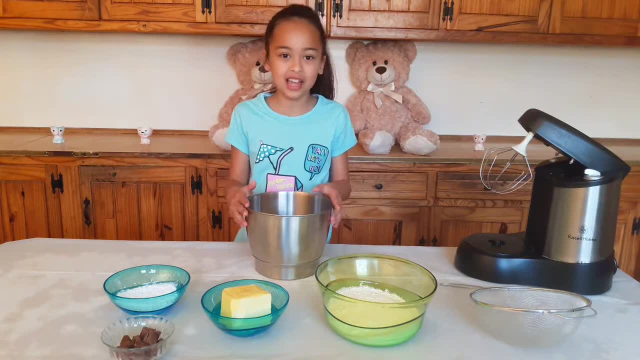 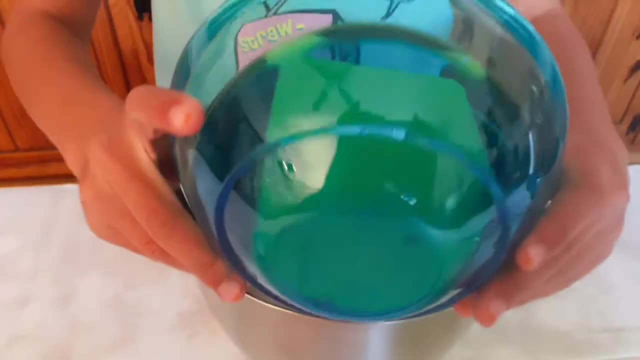 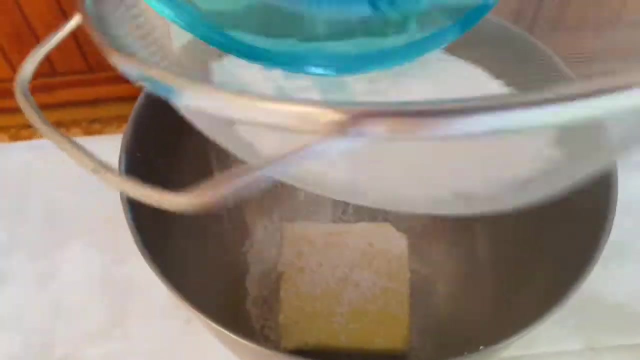 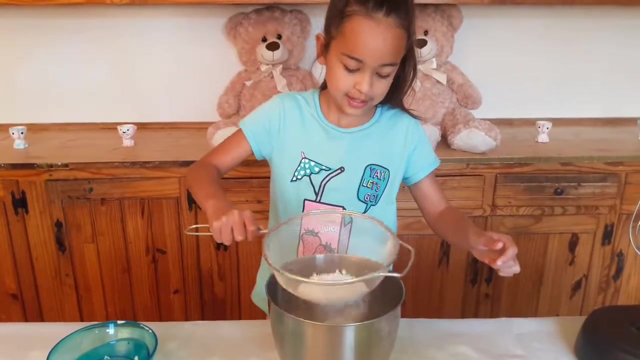 Then you will need your mixing bowl and combine your icing sugar And your butter together. Now I'm popping my butter into the bowl And sifting my icing sugar in there as well. Sifting, sifting, sifting. Ooh, there we go. It's like snowflakes. 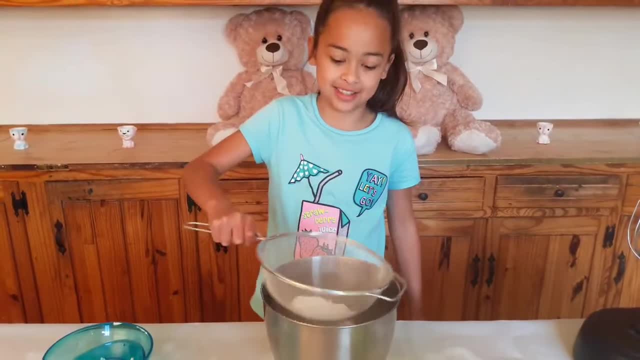 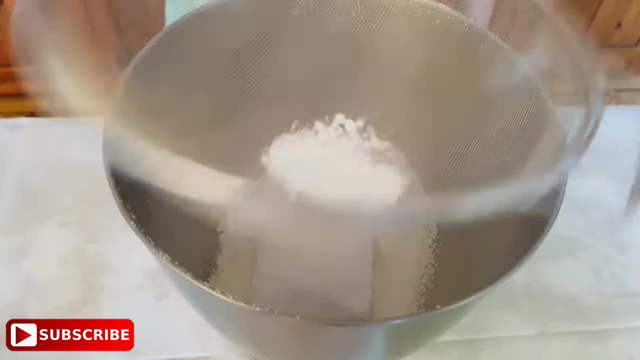 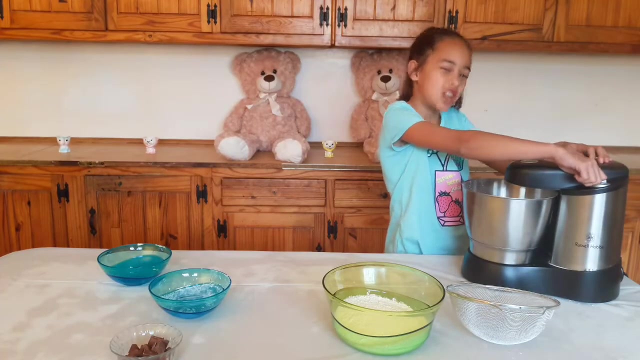 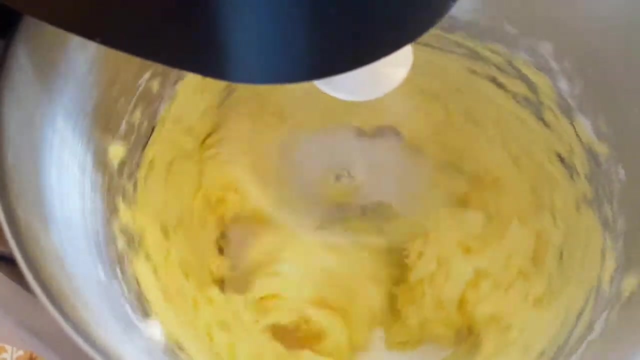 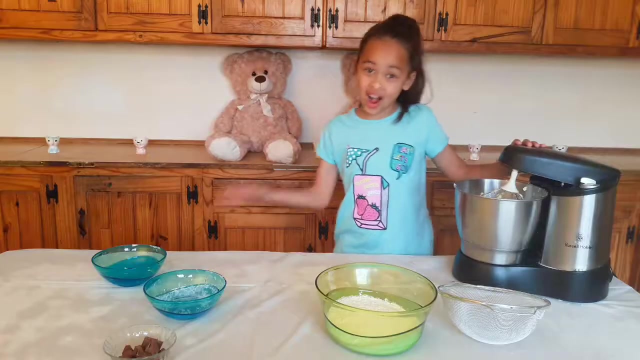 Coming down onto the butter Butters are ours, and icing sugar is for snowflakes, So almost done. Okay, that looks good. Now we will start the engines. Make sure you mix this until it's nice and creamy. Okay, guys, now it's time to get this baby out. 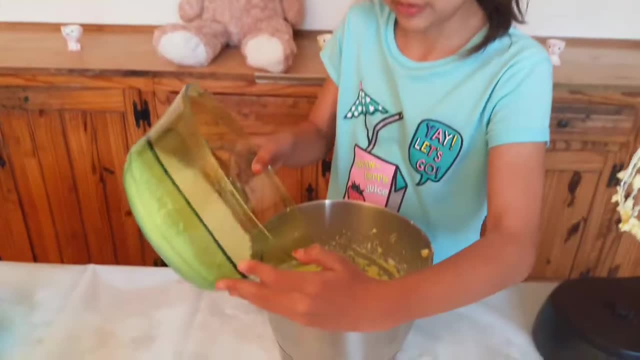 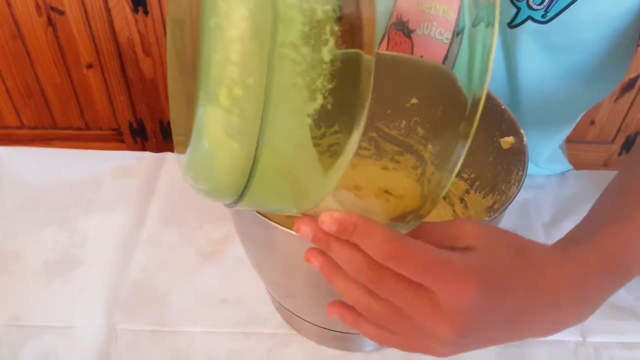 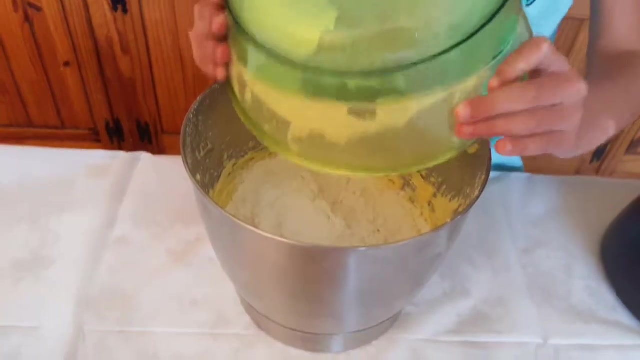 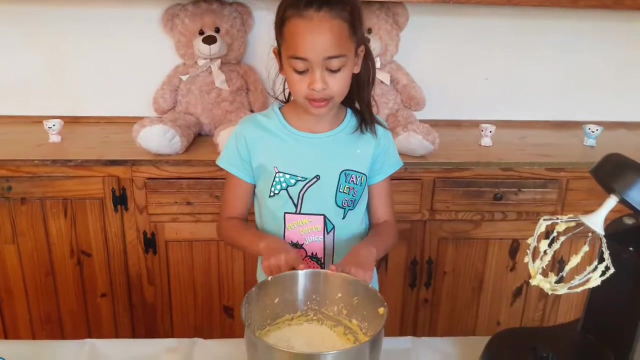 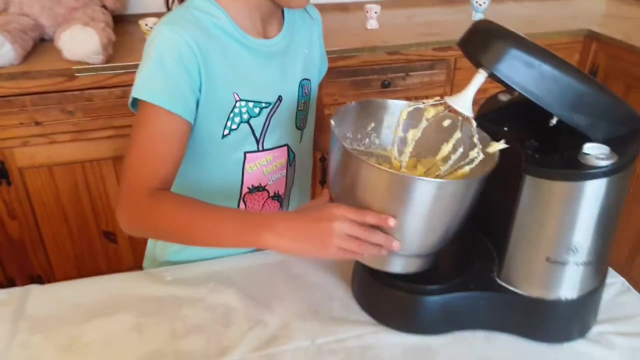 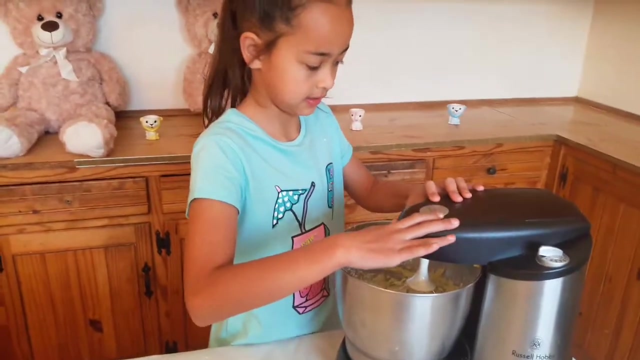 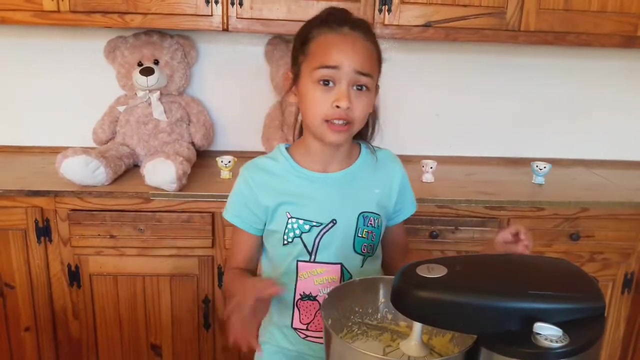 Now it's time to add in the flour: Slowly, slowly, slowly Go. What's this? There we go. Time to pop this back to the mixer. Okay, you guys might want to take this slow, Otherwise you're going to have a flour explosion. 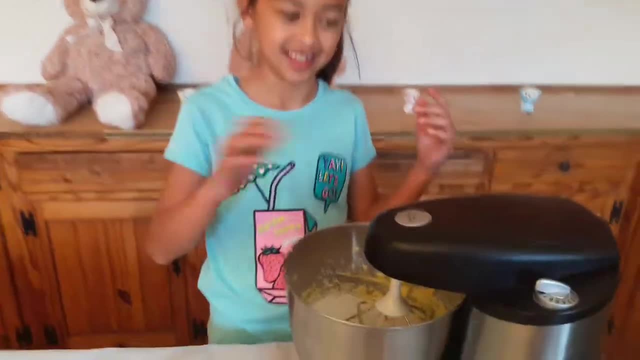 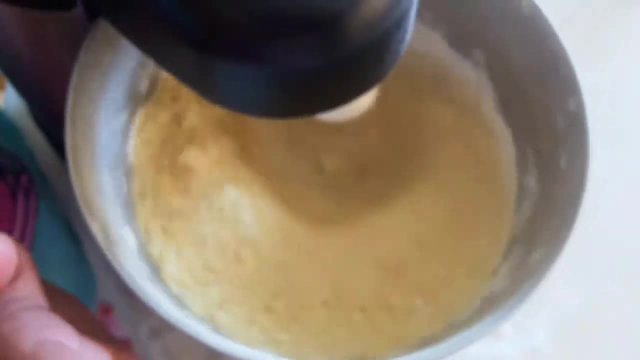 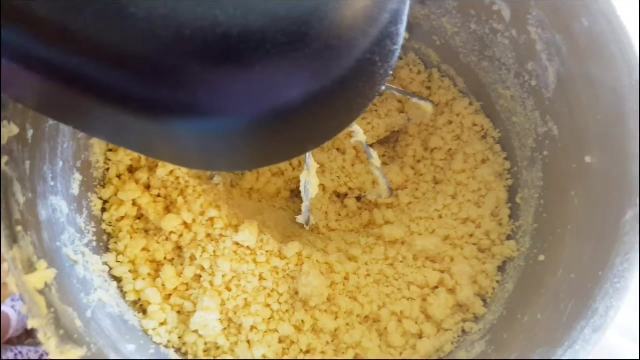 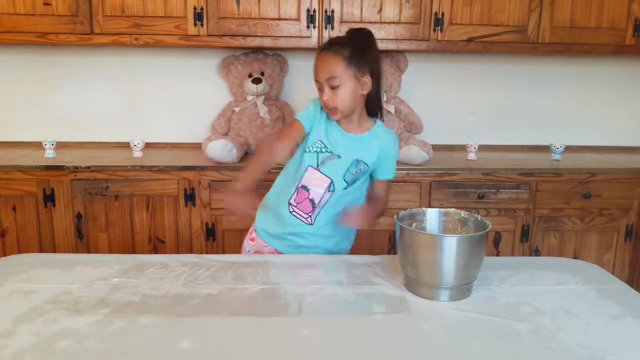 Like on a snowy day, So I'm going to take it slow. Ooh, It's starting to look like a Christmas, you guys? Okay guys, that looks awesome, Okay guys. so now what you want to do is put your cookie dough onto some cling wrap. 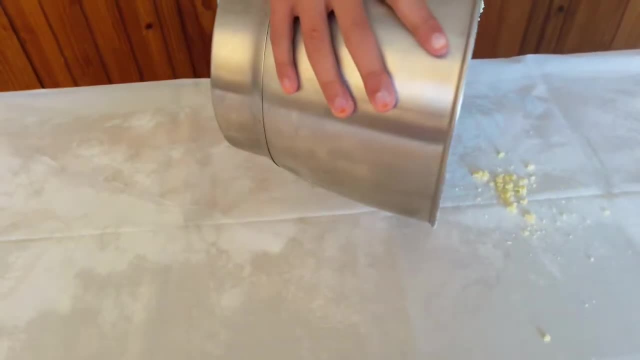 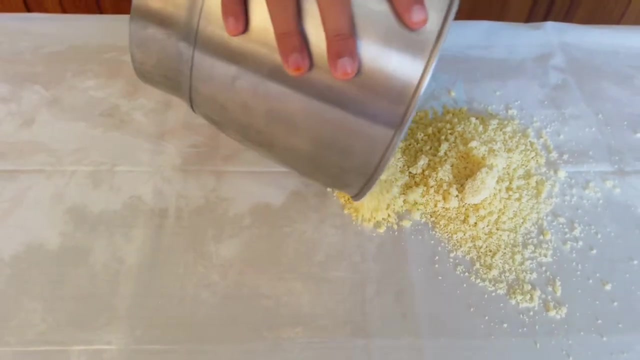 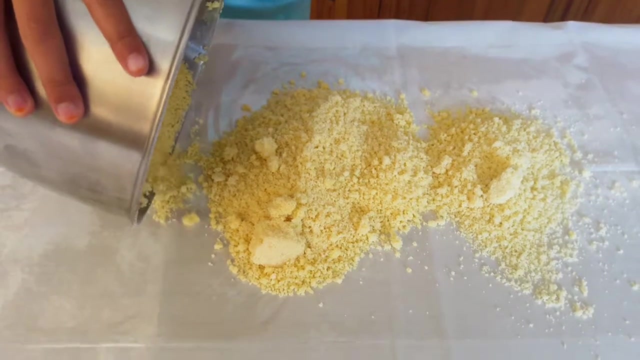 Okay, so I'm pouring this down. You guys might want to be careful, but I'm not being careful. I'm trying to be very careful. Okay, try not to get all over the top. Okay, that's good, Good. 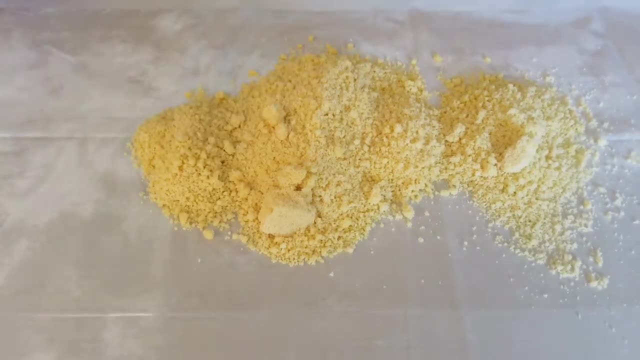 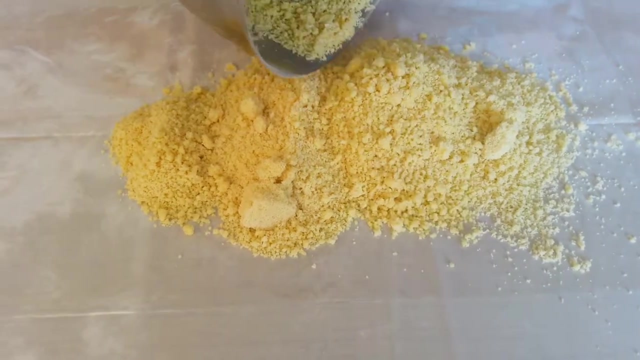 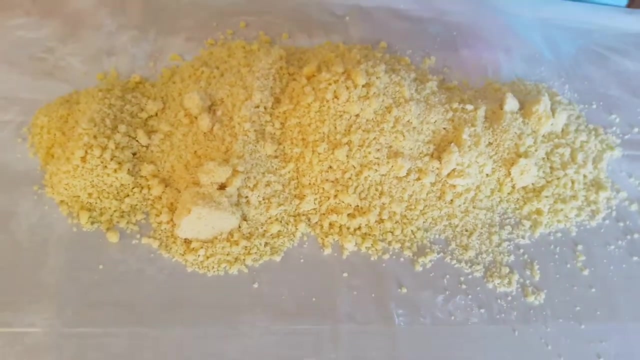 Put your cookie dough on top. Oh good chunks are there. Look, there's some over there. Let's see, Oh, some over here. Okay guys. so after I finish doing this, I'm going to wrap it up into a rug and pop it. 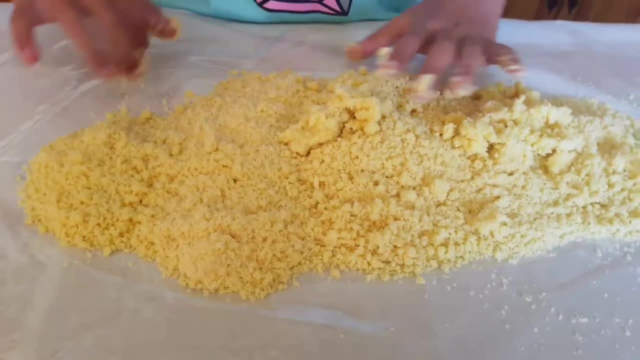 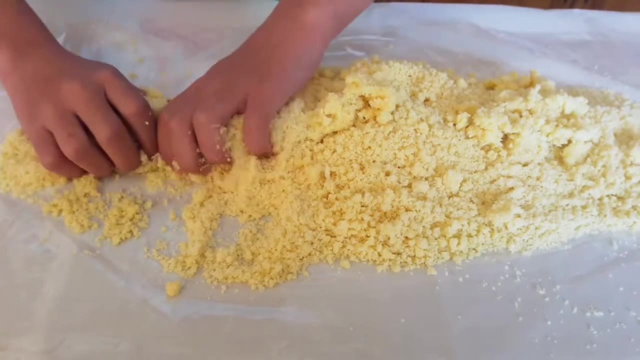 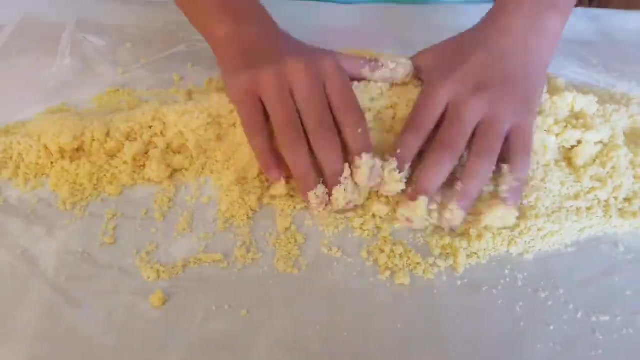 into the fridge and cool it down. Okay, guys, so now we're going to start putting it into the rug. this feels so cool, you guys. It's like a little boundary wall. I'm just going to squish a little, so it's fun. 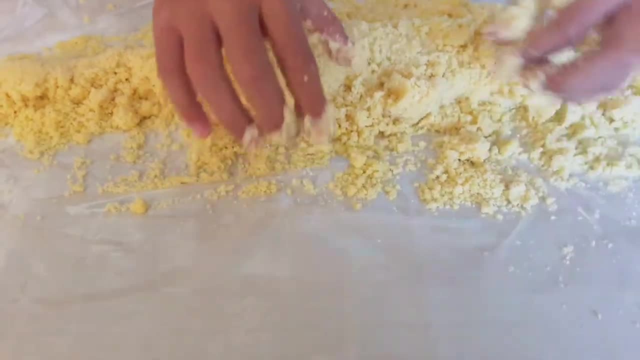 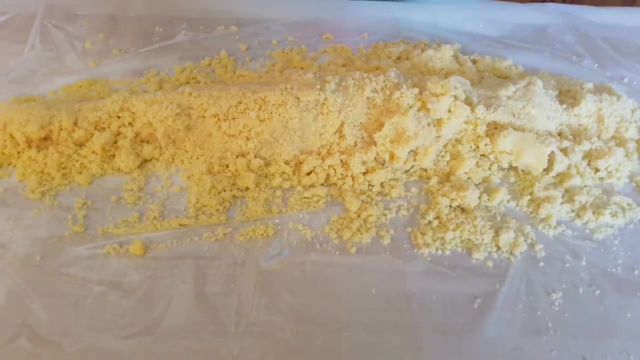 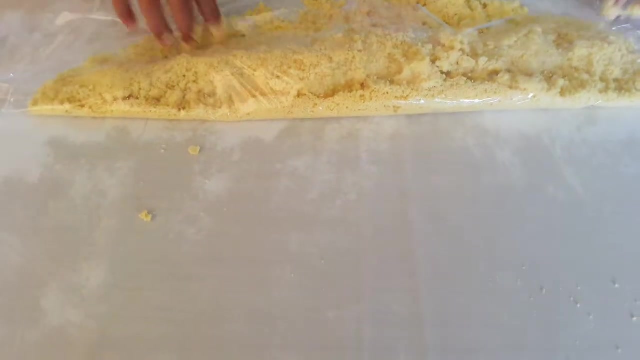 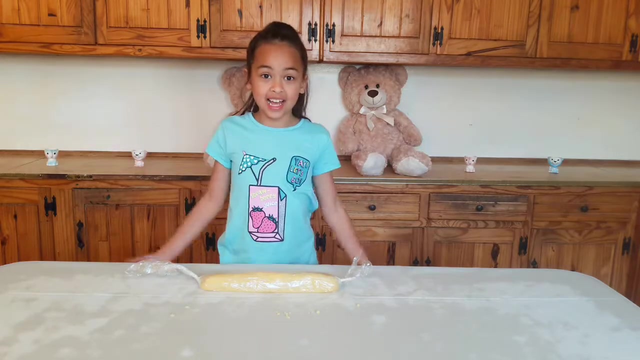 Okay, guys, I don't think this is working out for me. If you want, you can squish it like this and then cut it, but I prefer to rather turn this. Okay, guys, when you're done, it should look something like this: 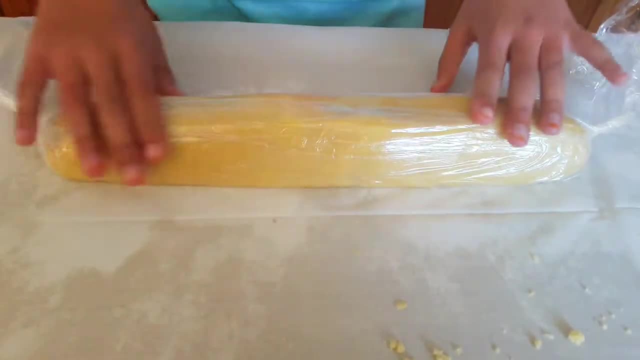 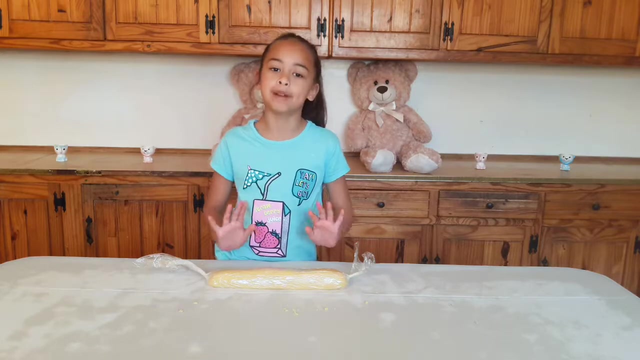 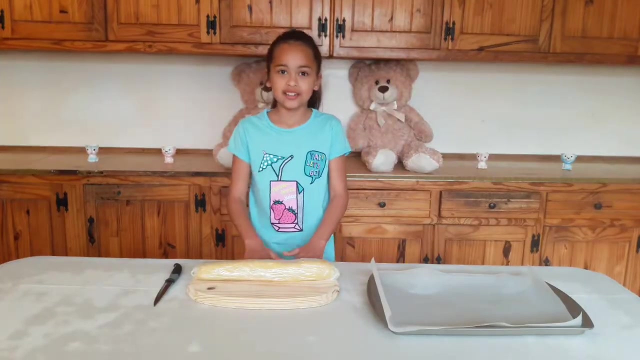 Beautiful, don't you think Beautiful? Okay, guys, we're done Shaping it like this. we're going to put it in the bread for 30 minutes. This will make it nice and firm. Okay, guys. so the cookie dough is nice and firm, so now we're going to cut into little bits. 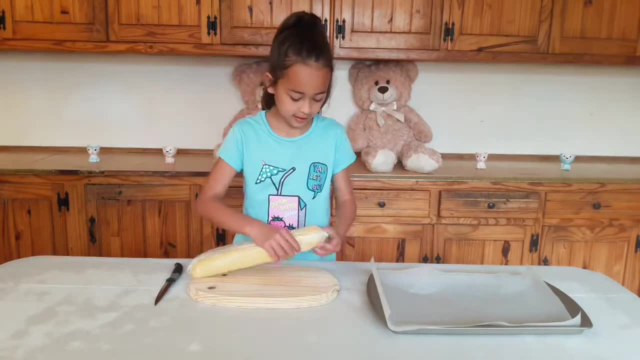 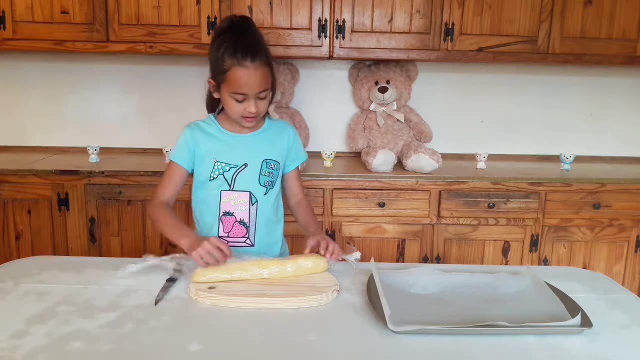 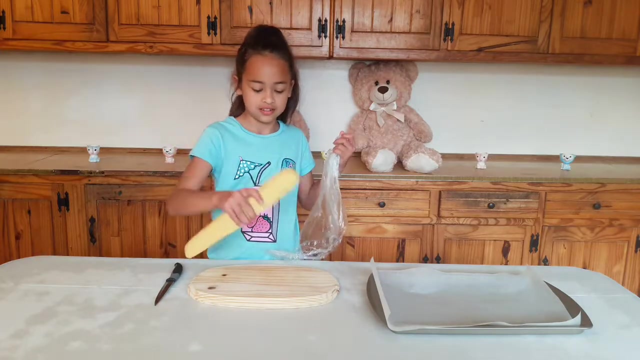 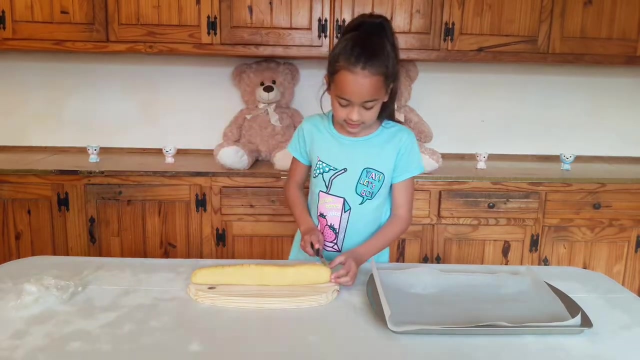 I popped onto the baking tray: Let's just unwrap this. It's like a present unwrapping it. A dough present. Dough, Dough, Dough, Do-shi-ya, Dough, Do-shi-ya. Okay, cut it. 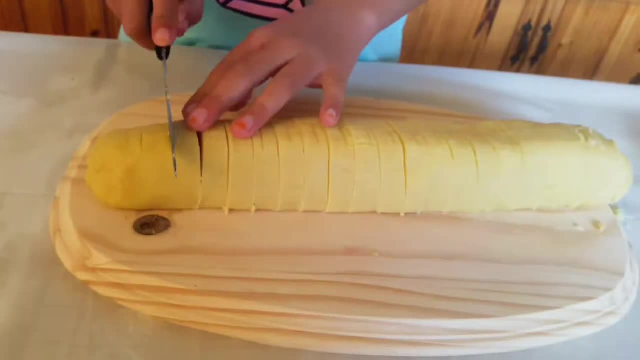 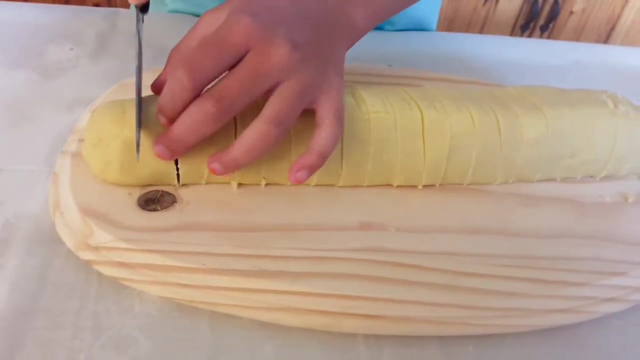 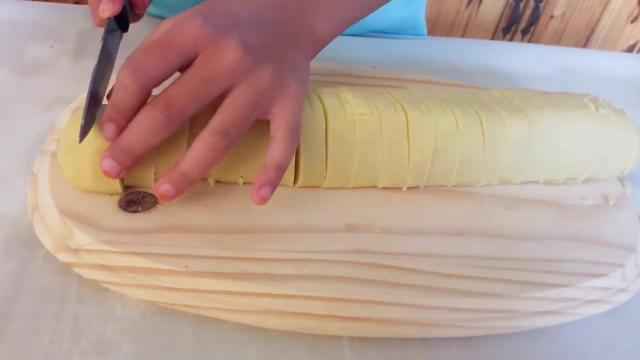 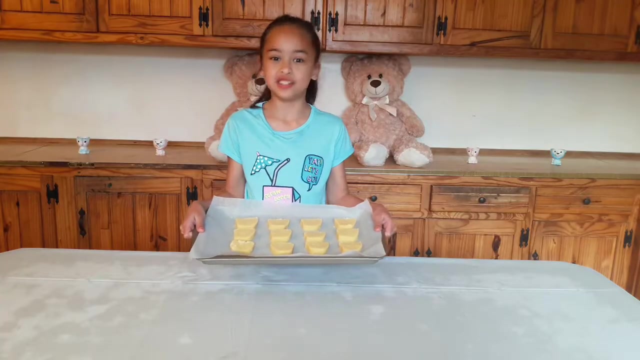 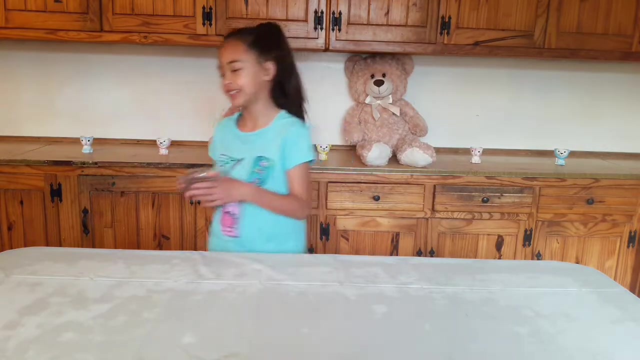 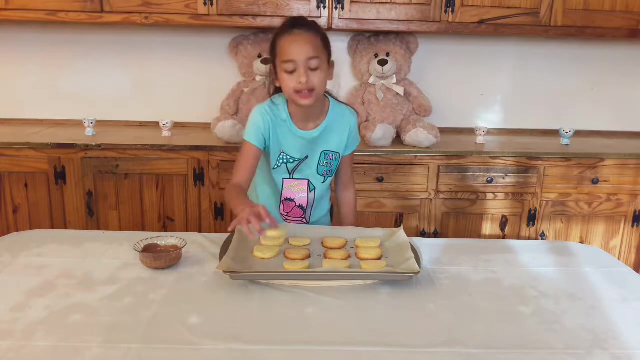 Also I want to help you with this part. Okay, guys, we're almost done with this end. Done with these into the oven. with the meat done, let's melt the chocolate. ok, guys, so the biscuits are done and they smell divine, so time to melt the chocolate. you can leave. 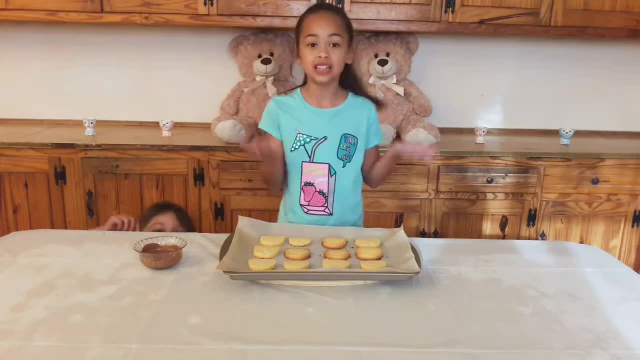 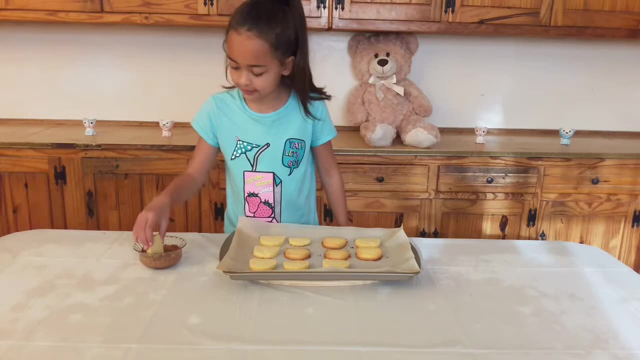 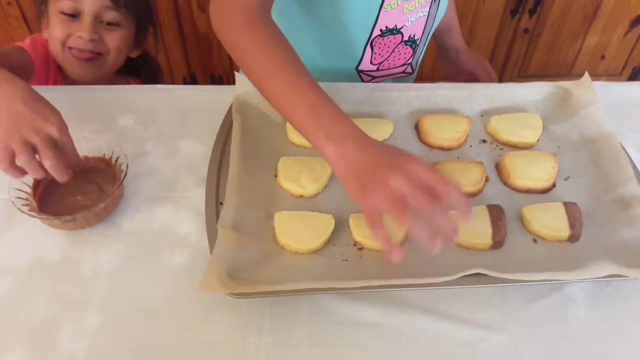 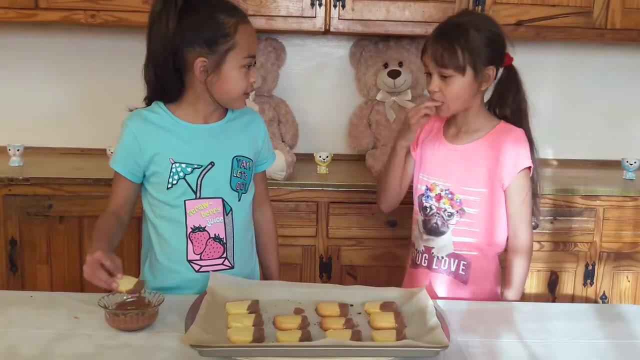 it as is, or you can dump them in the chocolate, because I really love chocolate, so let's go dump it. that looks so good like an artist. let's dump all the biscuits in the chocolate, let them dry and enjoy. what do you think of the biscuits? they look amazing. it's very. 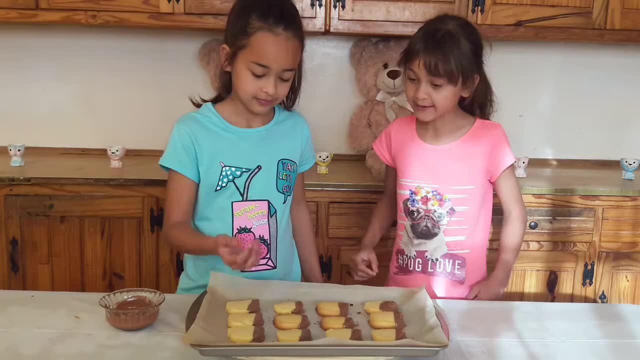 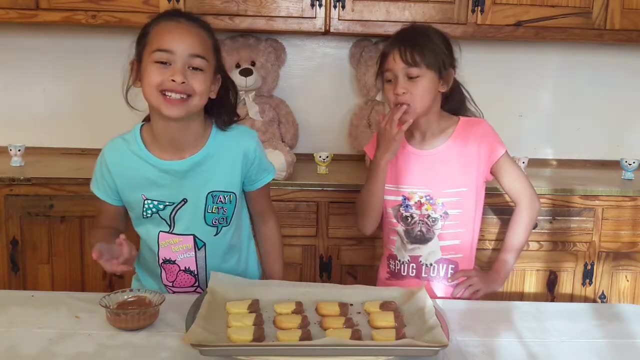 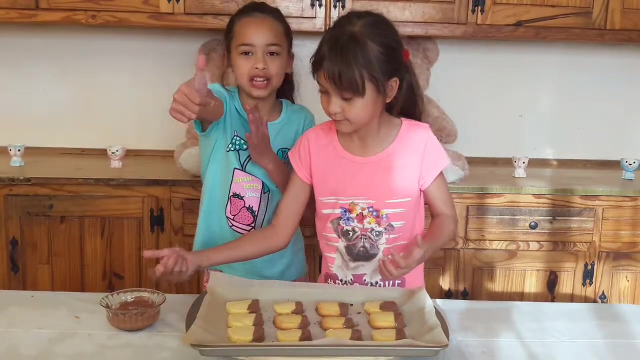 good. I love chocolate and that's why I like cookies, all the biscuits, and I love chocolate and my biscuits, biscuits and chocolate. Bye guys, hope you enjoyed this video. if you did, smash that like button, don't forget. 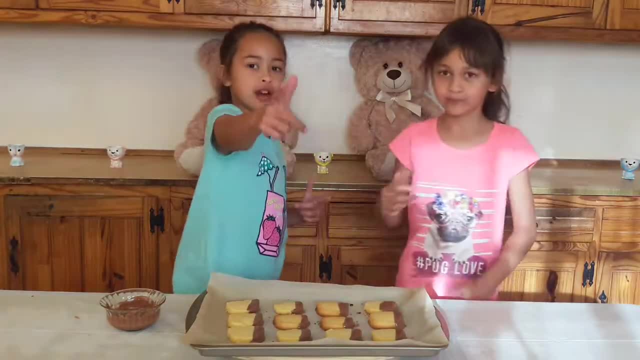 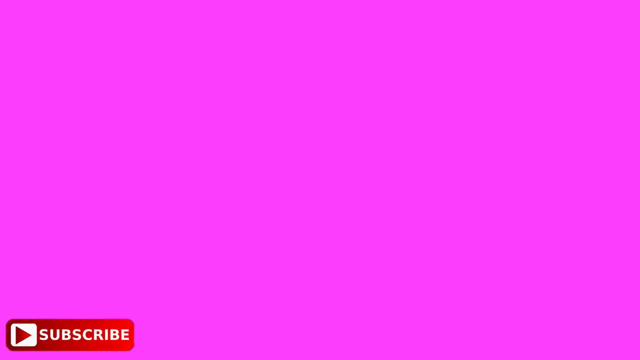 to like, comment and share. also, don't forget to subscribe. hit that notification bell. we'll see you guys next time. bye, Bye, Bye, Bye.